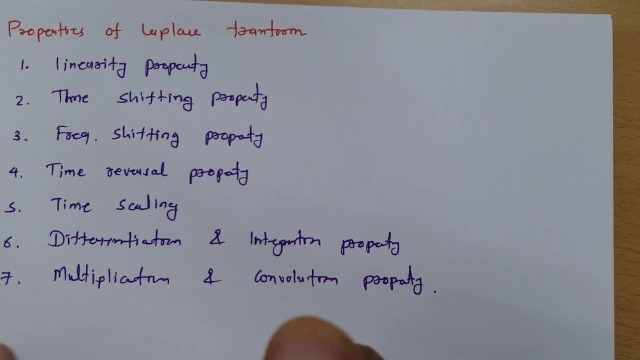 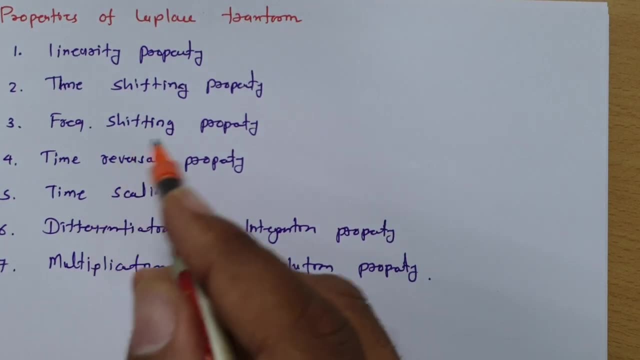 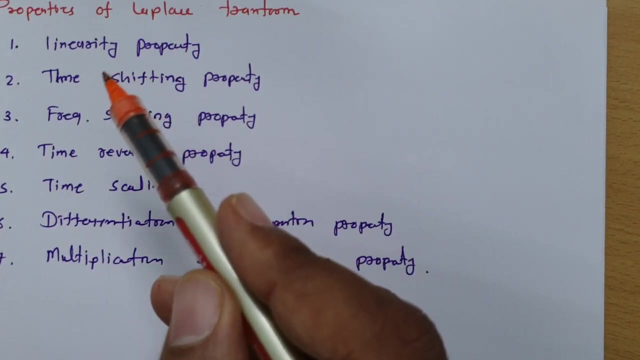 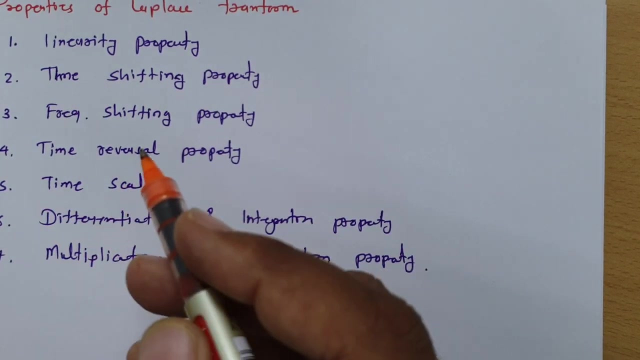 Welcome to signal and system lecture series Here in this session I'll be going to explain properties of Laplace transform. Now see, in this session I'll just define all those properties And for individual properties I have made separate session how we can derive those relations. So I have made separate session based on how we can derive all those properties. So that is what individually. 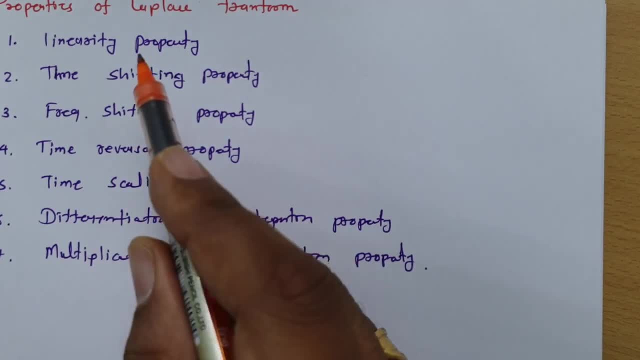 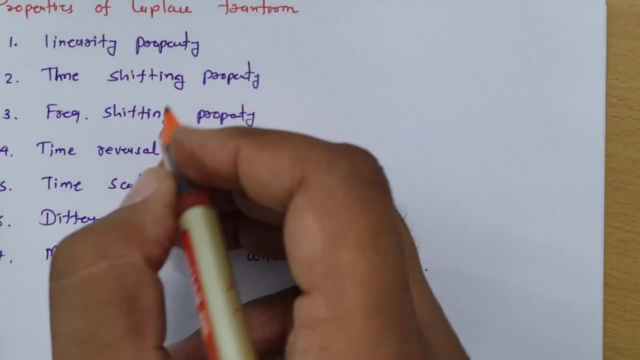 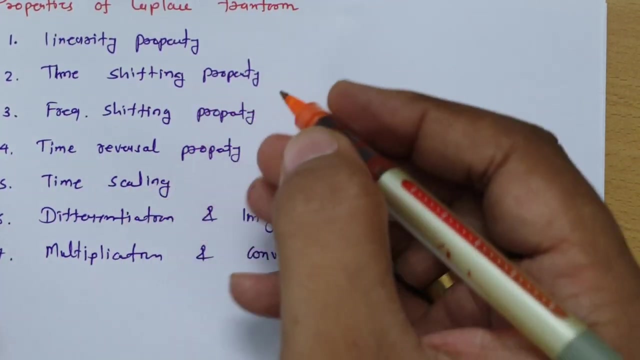 I have made. Here I'll be explaining properties of Laplace transform with their basic definitions. So let us have first property, that is linearity property. Now see to explain linearity property. it should follow superposition theorem. So if we have two signals, x1 and x2, and if you 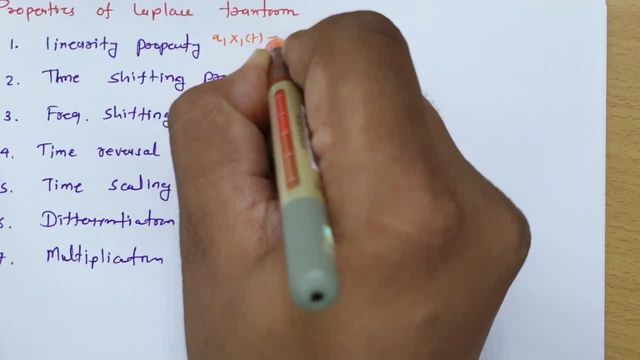 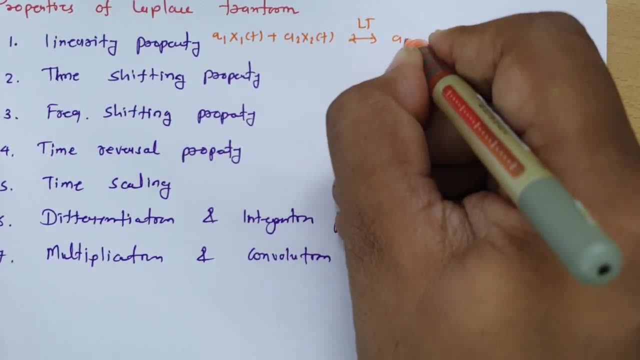 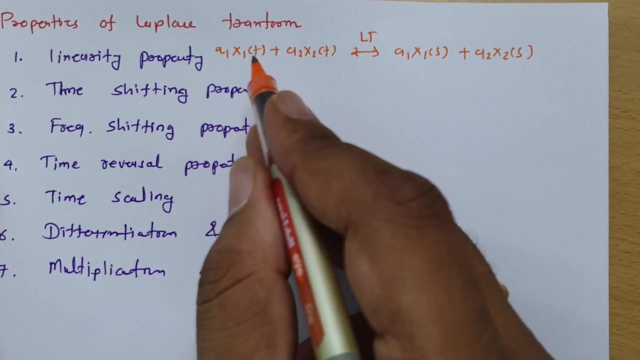 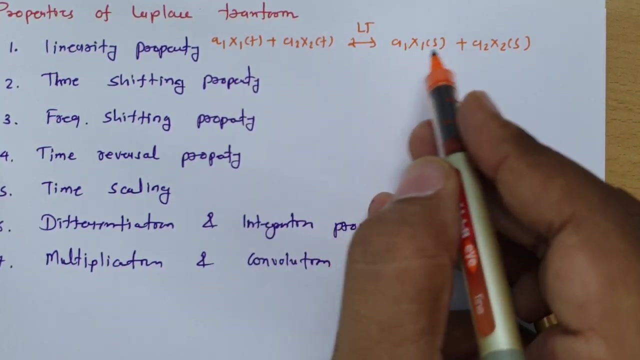 do Laplace transform of a1- x1 t plus a2- x2 t, then that Laplace transform that should be a1 x1 of s plus a2 x2 of s. So this is what property of linearity for Laplace transform. where x1 is Laplace transform of x1, s is Laplace transform of. 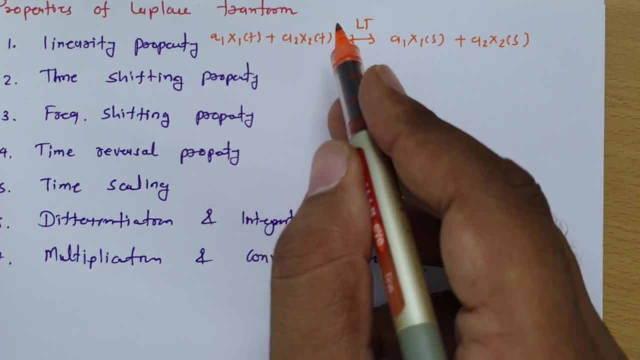 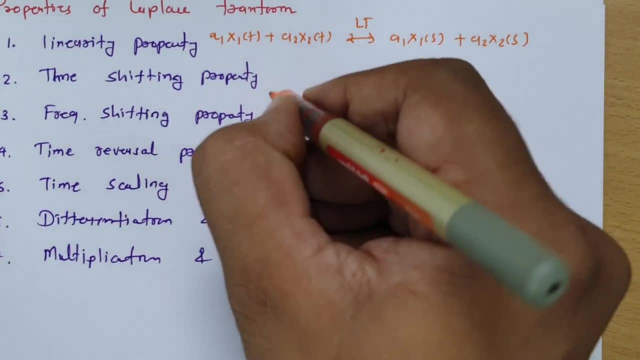 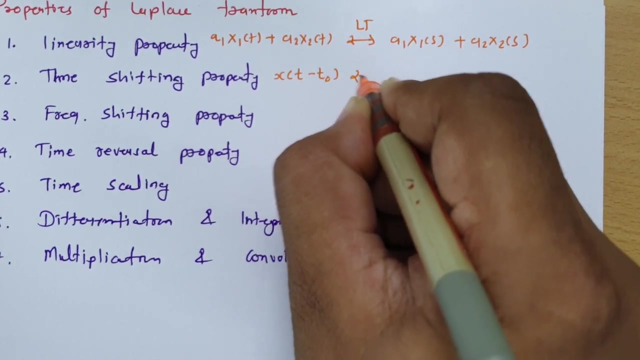 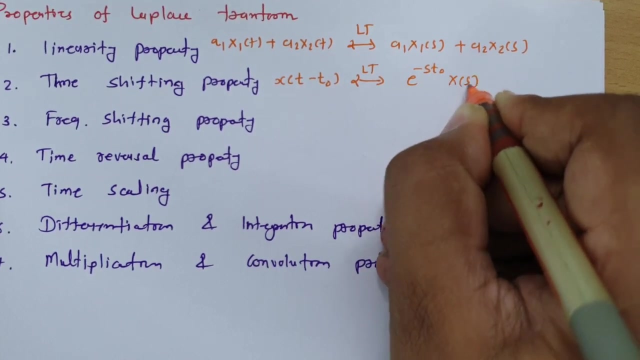 x1 of t and x2 of s is Laplace transform of x2 of t. So this is what linearity property, time shifting property. So if you have any signal x of t and if you shift it by time t minus t0, then Laplace transform of that has to be e to the power minus s, t0, x of s. where x of s is Laplace transform of x of t. 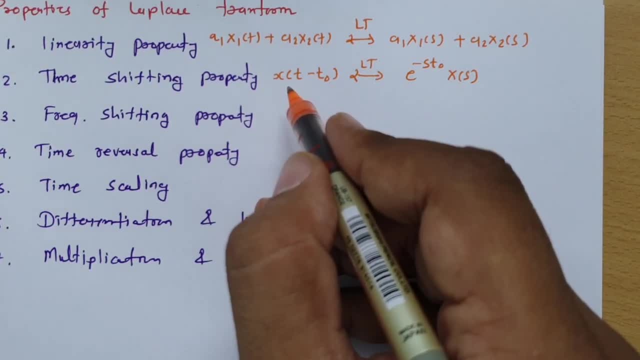 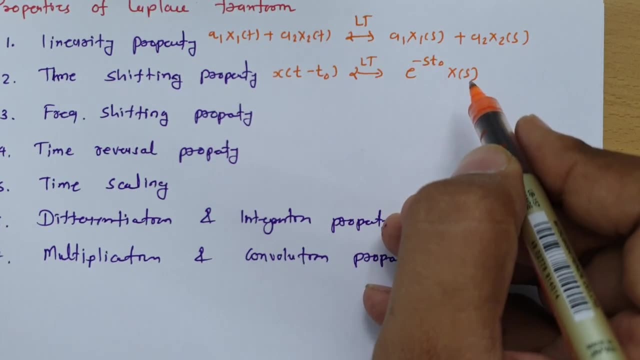 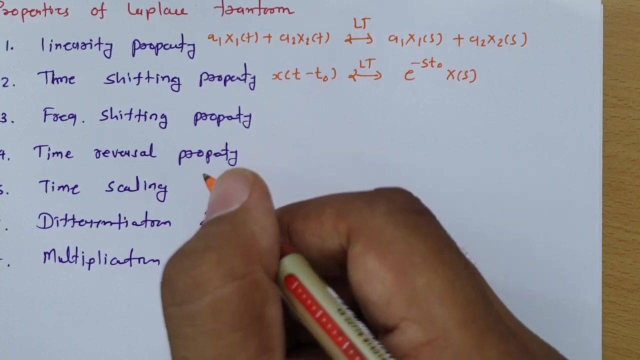 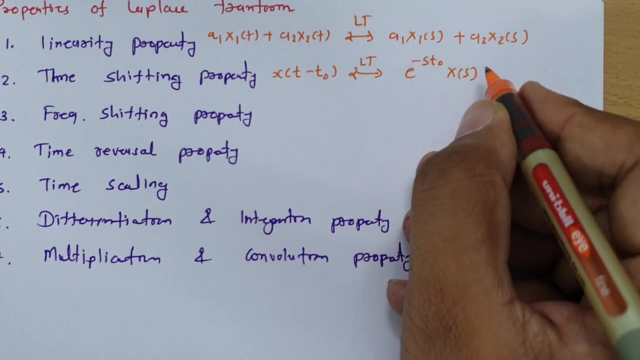 So if you shift x of t by x of t minus t0, then Laplace transform will be e to the power minus s, t0, x of s. Now let us see frequency shifting property. So when we shift frequency, so in that case you will be shifting frequency domain means x of s domain. 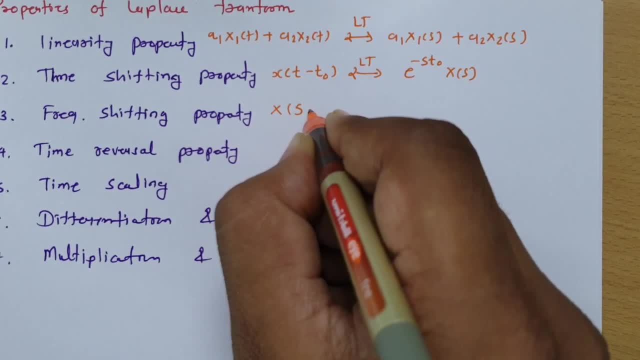 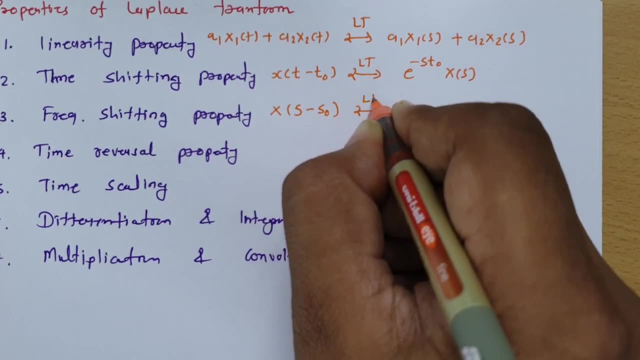 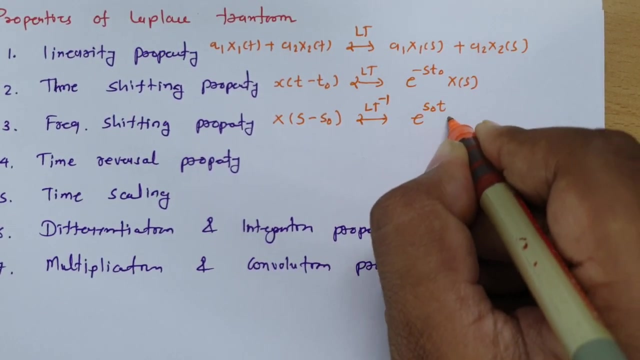 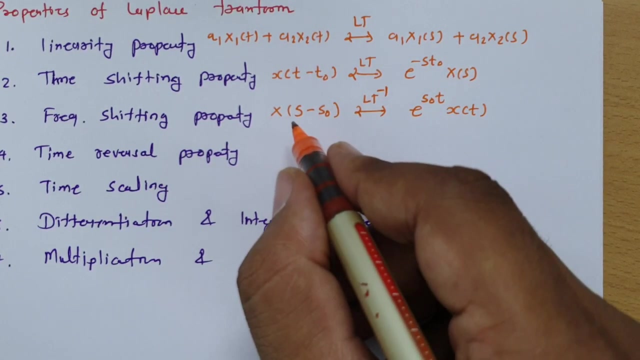 So if you have frequency domain x of s and if you shift it by x of s minus s0, then inverse Laplace of that will be e to the power s0 t. x of t means if you multiply e to the power s0 t with input signal, in that case it will be shifting frequency by x of s minus s0. 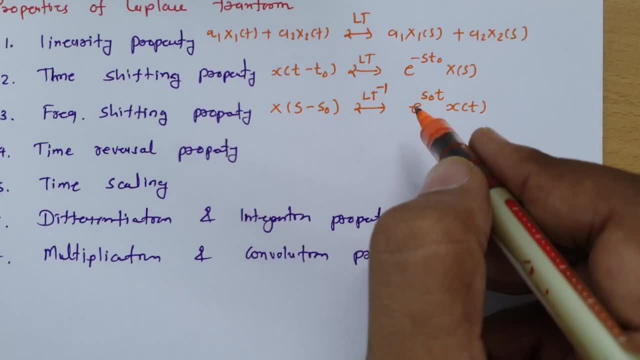 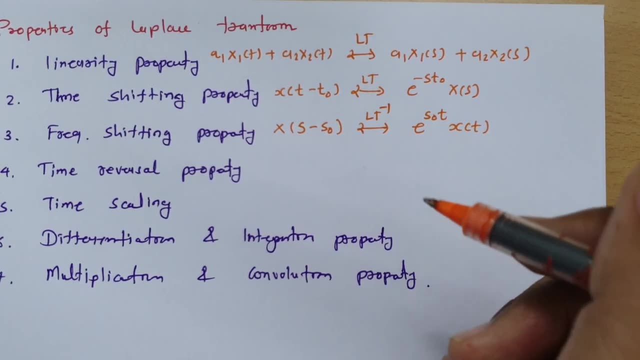 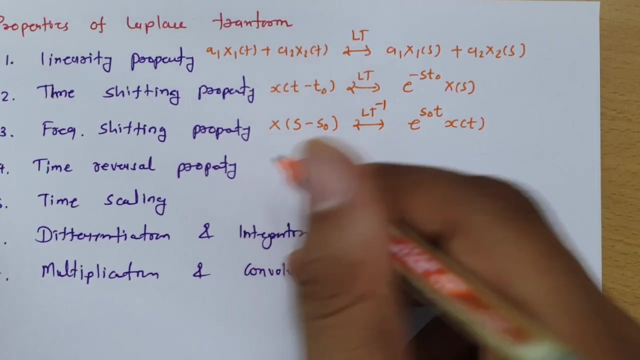 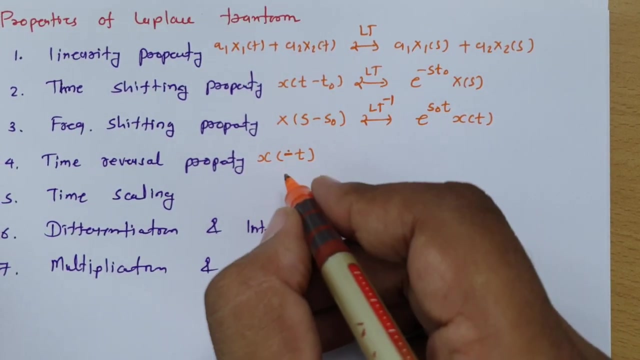 So, ultimately, frequency shifting means what you will have to multiply e to the power s0, t to shift it by s minus s0.. See, this is how frequency shifting is possible in Laplace transform. Now, next is time reversal. So if you reverse the time, so what I do is I will be reversing it by taking t is equals to minus t. 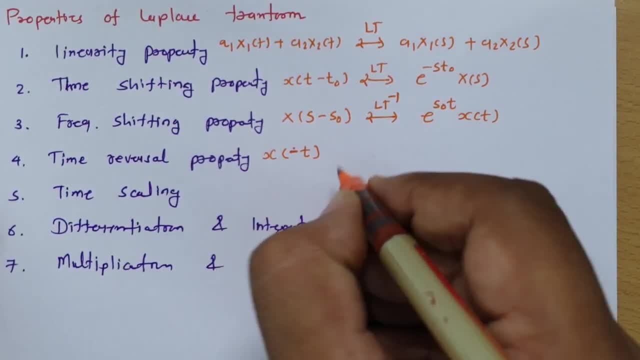 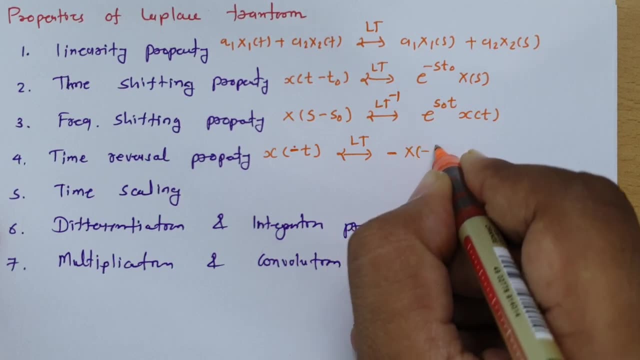 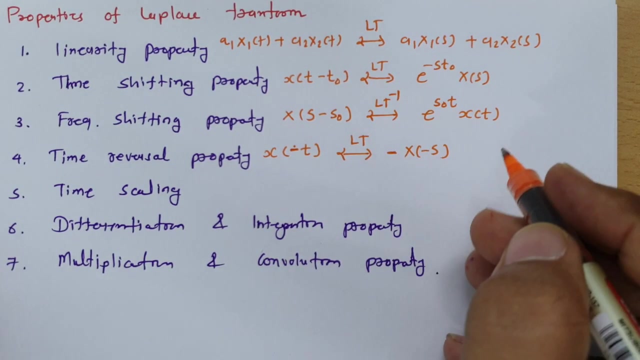 So there will be time reversal. So if you do time reversal in Laplace transform, in Laplace transform, you will be observing it will be minus of x, of minus s. So this is how time reversal is happening in Laplace transform. Now, next is time scaling property. 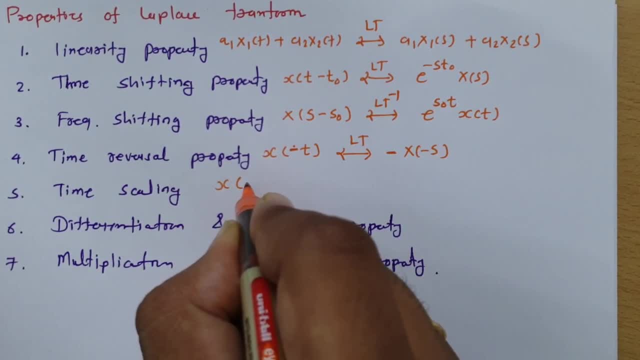 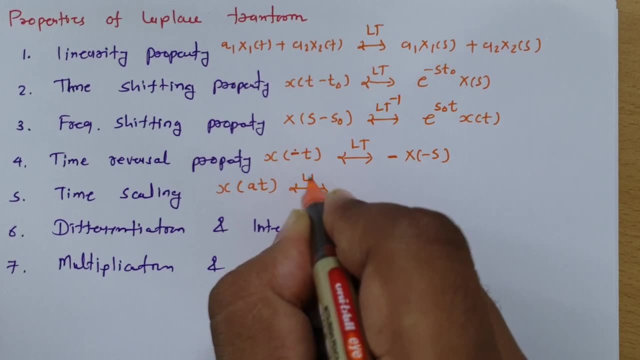 So if you scale time like see if you have x of t, and if you are scaling it by factor a, by multiplying a with time, t, in that case in Laplace transform you will be observing it will be 1 by a, x of s by a. 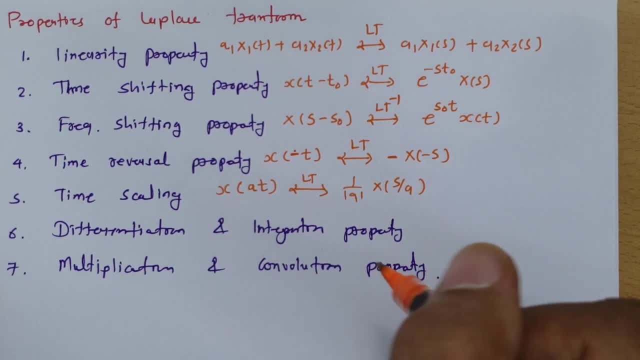 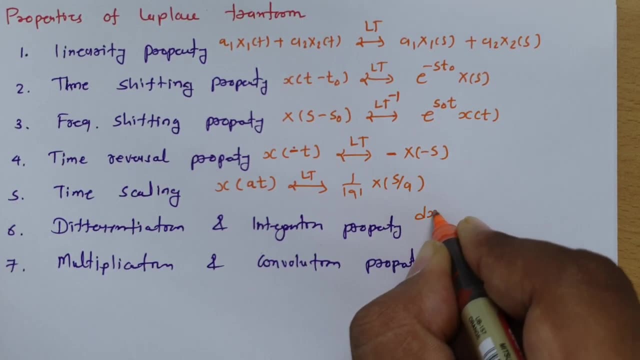 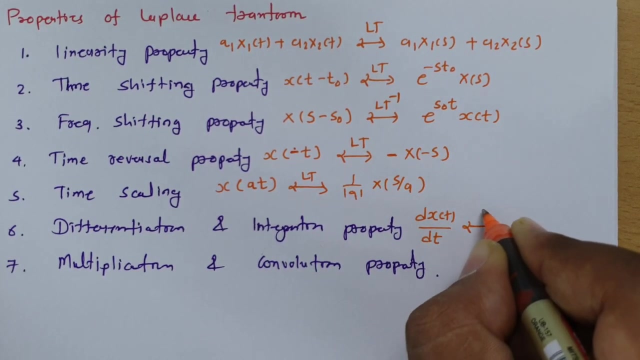 So this is how time scaling is happening Now. differentiation and integration property. So see, first I will explain you differentiation property, Where, if you have differentiation, So if you have differentiation of x of t with respect to time, and if you take Laplace, transform of it, in that case you will have to multiply s with x of s. 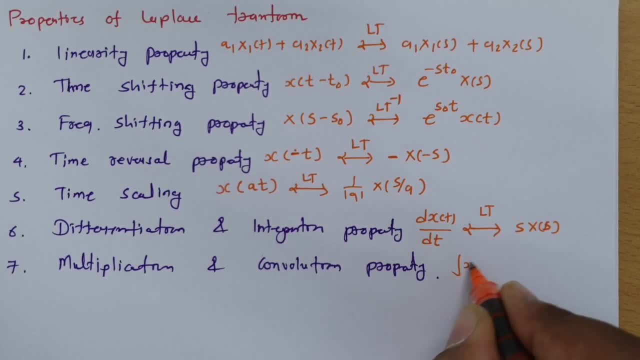 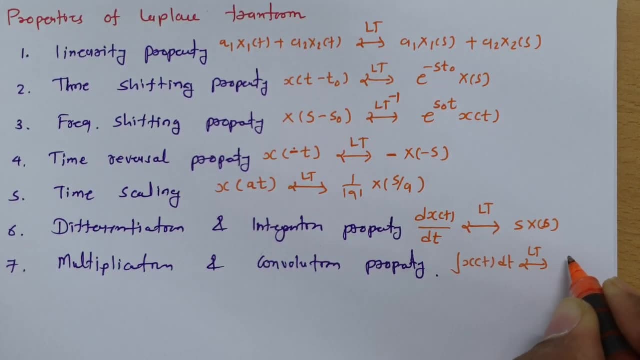 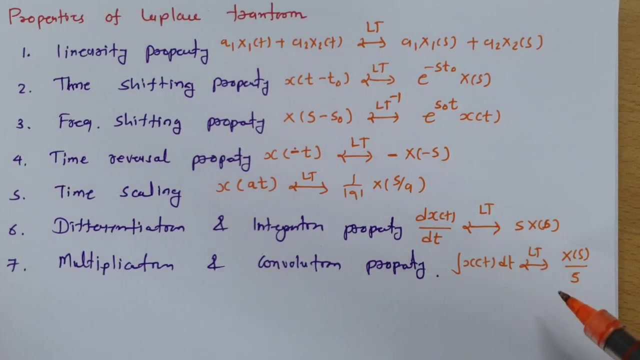 And for integration. if you have integration of x of t and if you take Laplace transform of it, then it will be x of s divided by s. So this is how integration and differentiation properties are there. Now, last property, that is, multiplication and convolution property.